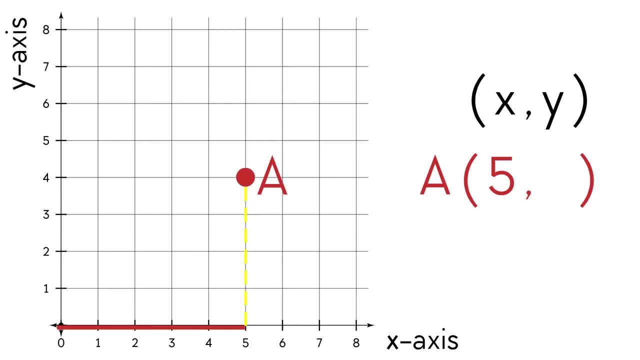 distance from zero. To do this we look at the left, to the y-axis, to find the point's vertical distance from zero. So the y-coordinate is 4.. So the ordered pair A is: Let's find the ordered pair for B. First. we find the x-coordinate, We look down at. 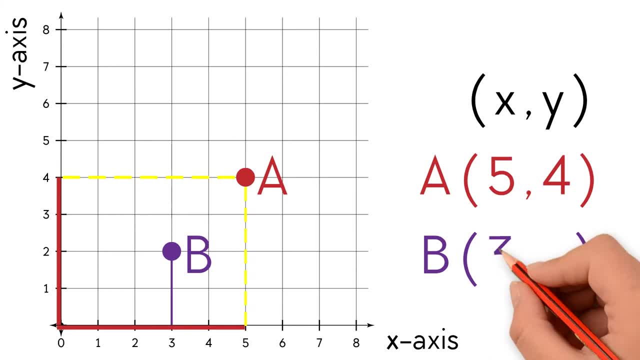 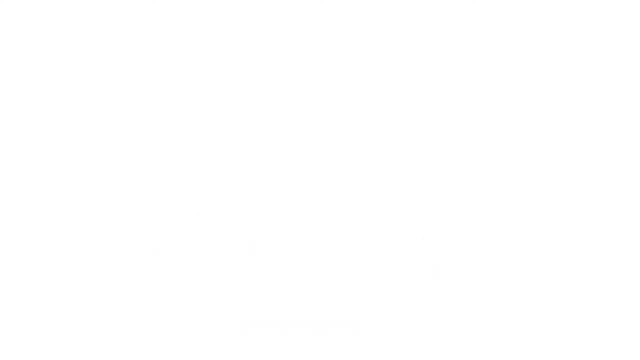 the x-axis and we see that the x-coordinate is 3.. Now let's find the y-coordinate. We look to the left and we see that the y-coordinate is 2.. So the ordered pair for B is: Let's do some more examples. 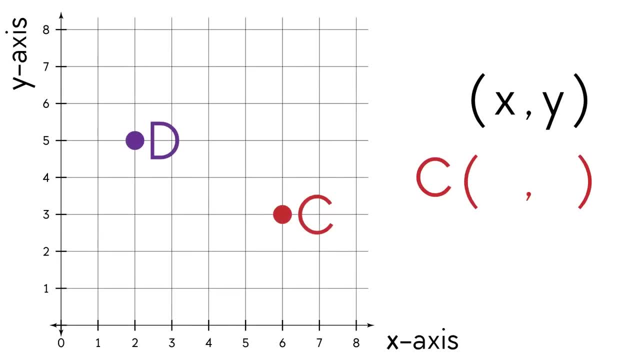 Find the ordered pair for C. First we find the x-coordinate. We look down to the x-axis and we see that the x-coordinate is 6.. Now we find the y-coordinate. by looking to the left at the y-axis, We see that the 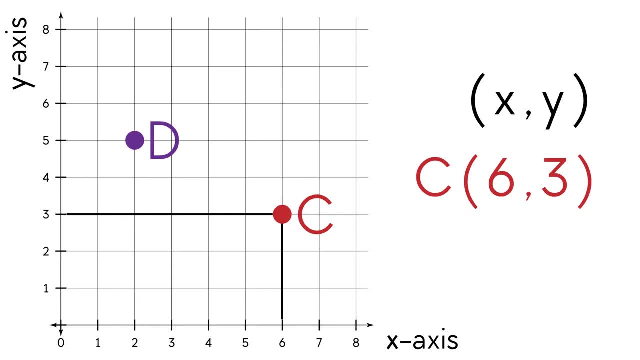 y-coordinate is 3.. So the ordered pair for C is Now. let's find the ordered pair for D. We start with the x-coordinate, We look down at the x-axis and we see that the x-coordinate is 2.. Let's find the y-coordinate. We look 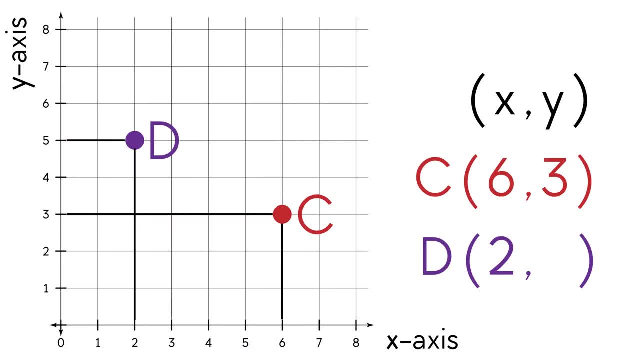 to the left at the y-axis, and we see that the y-coordinate is 5.. So the ordered pair for D is Now. let's try to plot ordered pairs. First. let's try to plot A. We start at the origin, which is where the x-axis and the y-axis intersect. We move right. 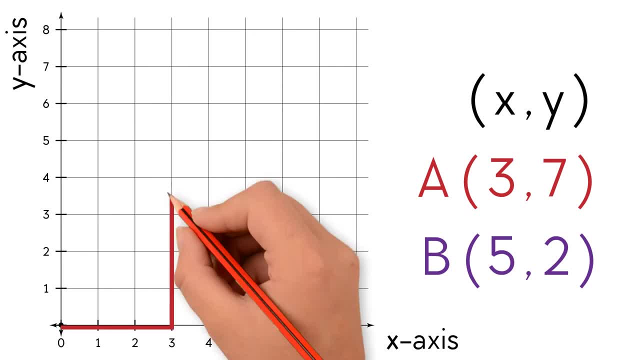 3 units and then up 7 units. Now we can plot and label the point. Now let's plot point B. We start at the origin and we move right 5 units. Then we move up 2 units. Now we can plot the point.